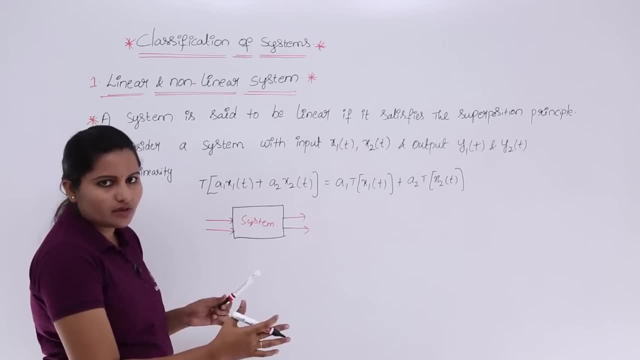 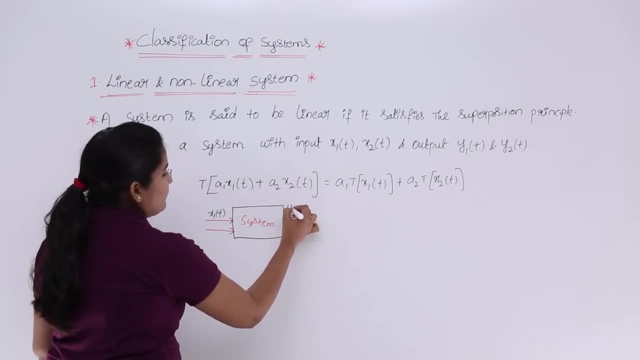 or any system. This is a. this is any a system with a particular response. If you are giving x 1 of t, then you are going to get y 1 of t. If you are giving x 2 of t, then whatever. 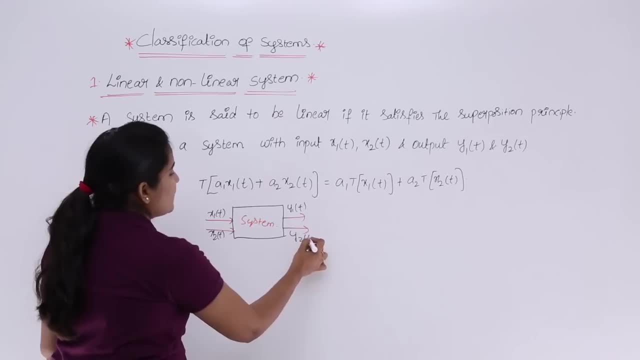 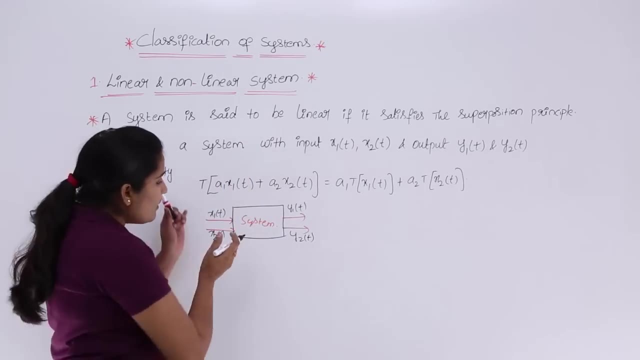 response we are getting that I am considering as y 2 of t. Now to To say this system is linear, then you need to satisfy this condition. That means of you, for example, first of all you need to give x 1 of t and you need to observe the 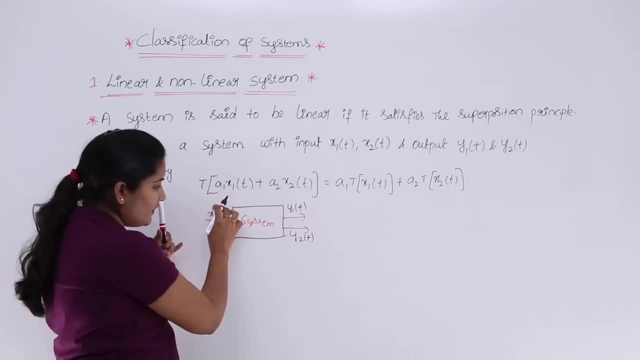 output, And second time after, after giving. after getting the response of first signal, you need to give x 2 of t and you need to get y 2 of t. Finally, you need to combine the responses. So that is, that must be equal to. So by at: 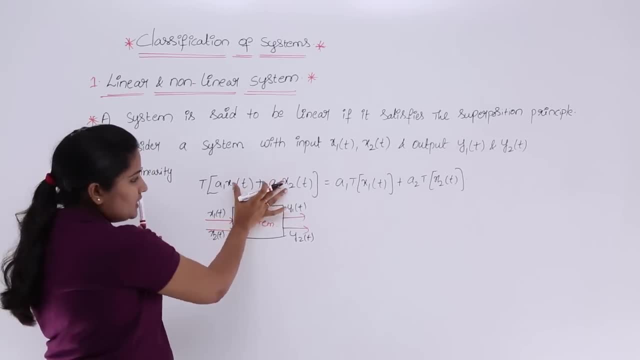 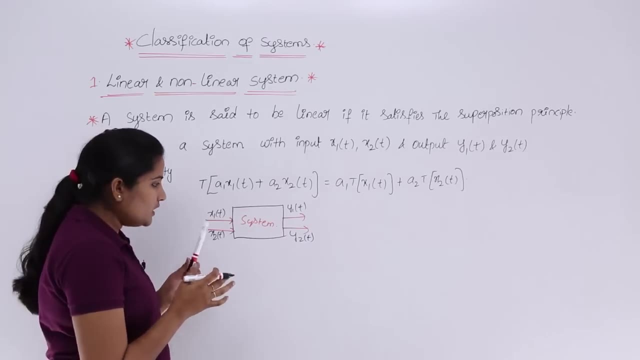 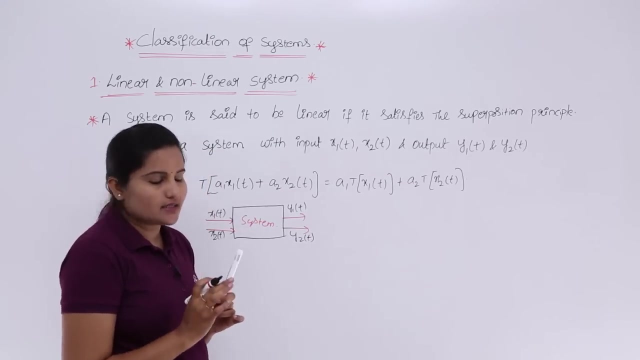 at the time, By the time of input itself. you need to combine two signals like this and you need to provide the output that must be equal to the previous added output. So here, so if this system satisfied that condition, so particularly that is said to be a linear system. To explain: 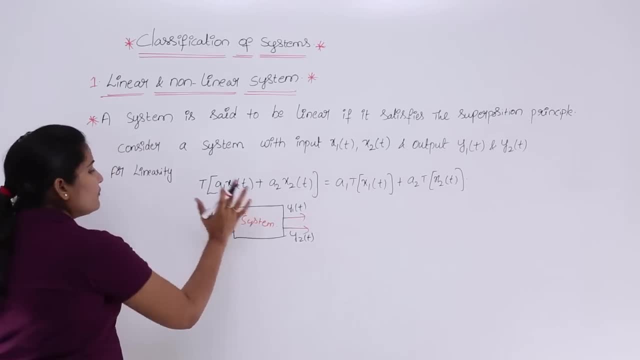 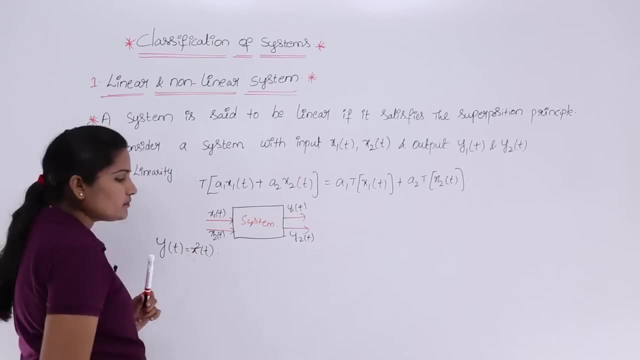 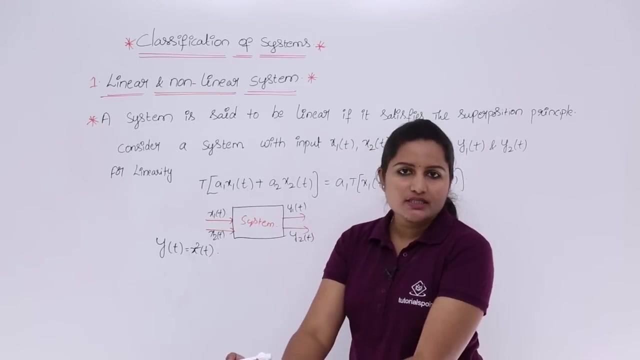 clearly. I am going to consider an example. so here, For example, this is a system with the response y of t is equivalent to x, x square of t. 3. treat this system is a squaring system. that means whatever signal we are giving to the system. 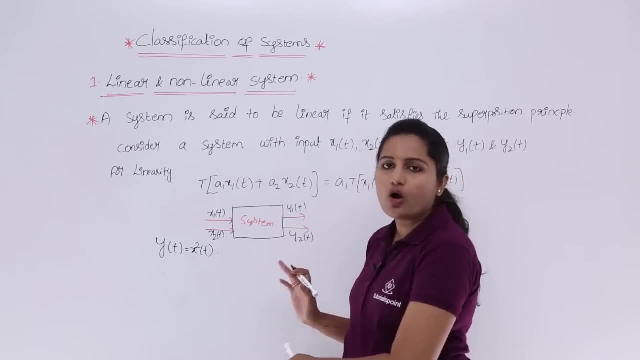 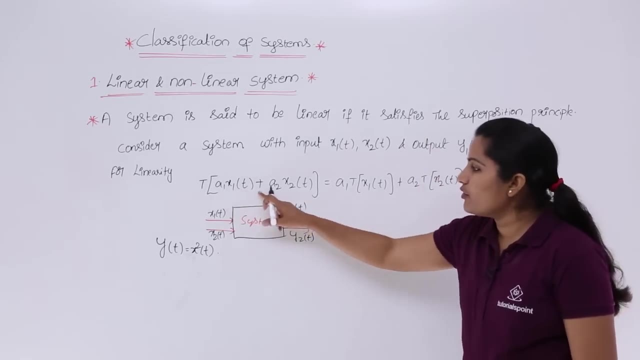 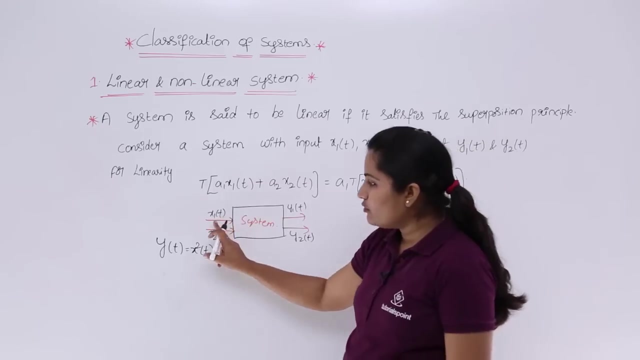 this is going to square that signal and giving output. So now I want to consider. I want to proceed individually, after that I want to combine the signal and I want to give as input. So first of all, for this system I want to provide only x 1 of t. that means t indicates. 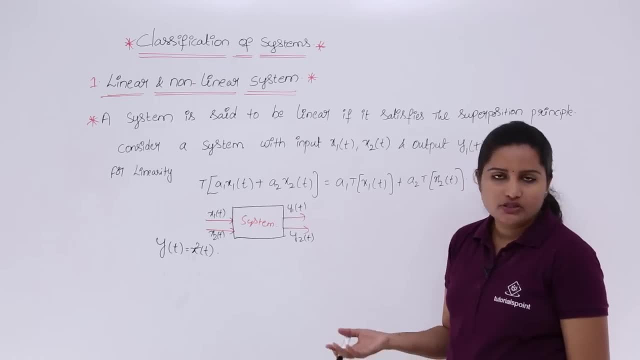 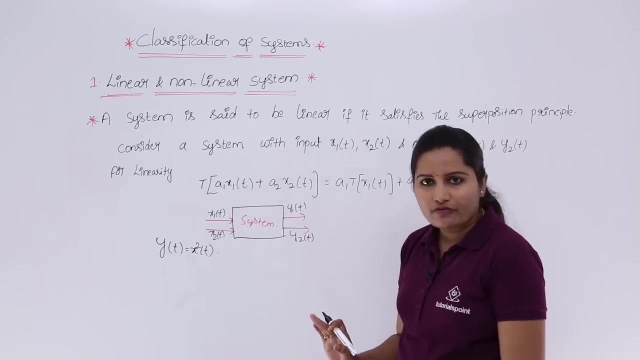 so transfer the signal, or response, you can consider like anything. So I want to consider this as so when this signal is transferred, transformed through that system, So like that I am going to consider here. So if you consider x, 1 of t first, then transform of. 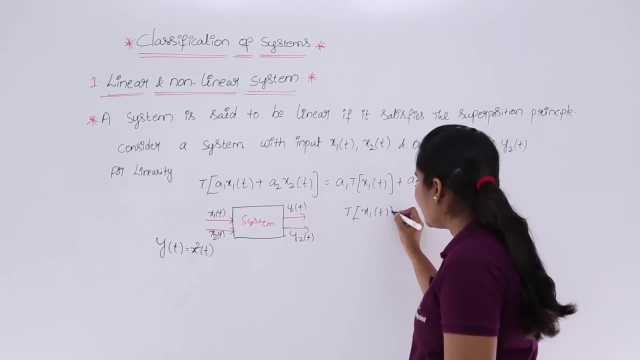 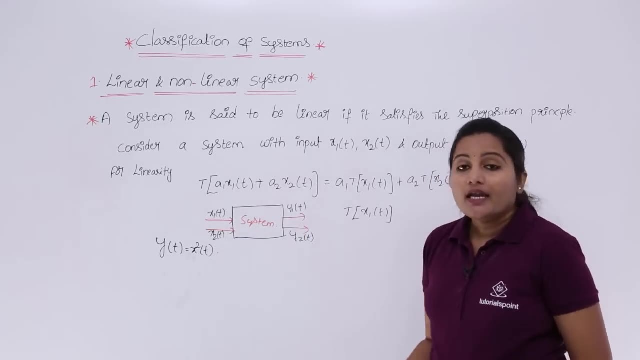 x 1 of t will become x: 1 square of t. why? because whatever we are giving the system, work is just to square. why? because they given In exam they will give. if a system with response y of t is equal to x square of t, then the system 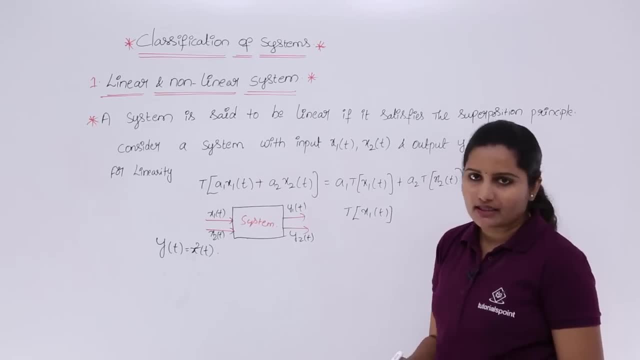 is linear or non-linear? they will ask like that. So now, according to the system response, whatever signal we are transforming from that system that is going to square, So x, 1 square of t will come as output. When you transformed your second signal, x 2 of t. 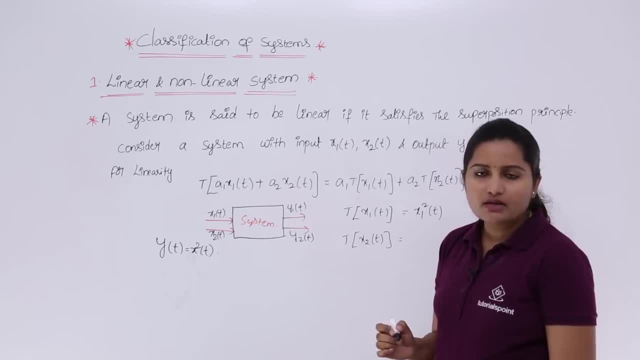 through this system, again, this system. what this system will do generally, whatever signal it is getting, it is going to square that signal. So you are going to get x square of t. then, third thing, what we need to do: initially, we need to combine the signal and you need to. 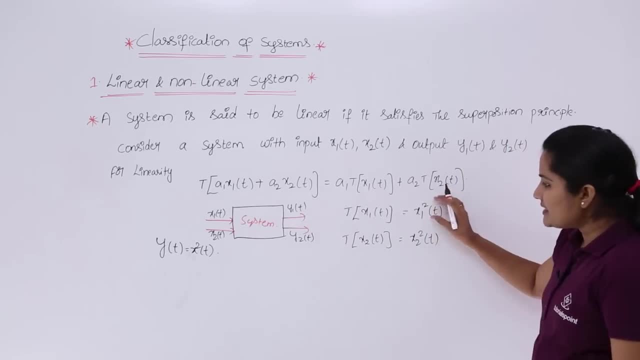 provide the output. So you can see this is a individual output. if you consider linearity, So you can consider a 1 x 1 of t. So you can consider a 1 x 2 of t. So you can consider: 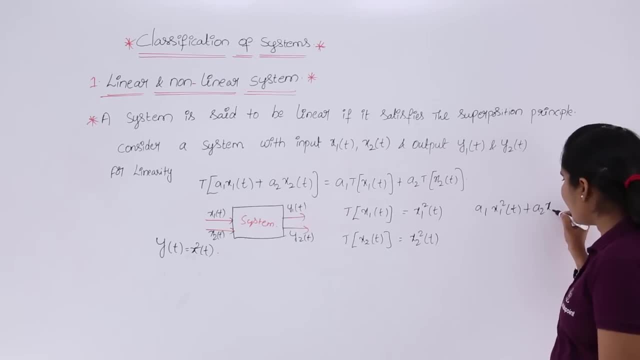 a 1 x 1 square of t plus a 2 x 2 square of t will be your right side part. So why? because transform of x 1 of t is x 1 square of t. transform of x 2 of t is x 2 square of t. So this will. 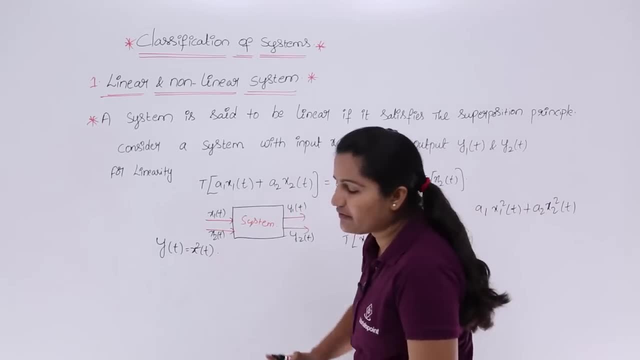 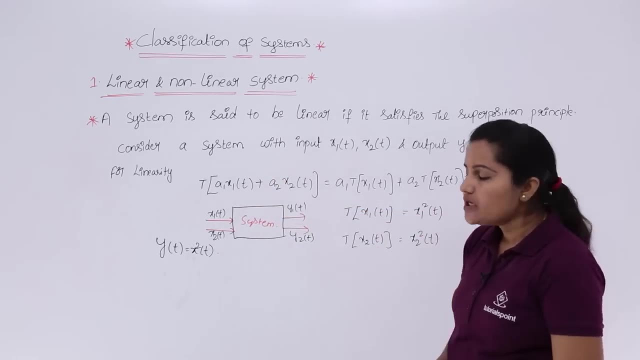 become like this for this system: with response y of t equal to x square of t. So now I want to check my LHS. that means combined signal input. So here if you transformed the combined signal input. So here if you transformed the combined signal input. So 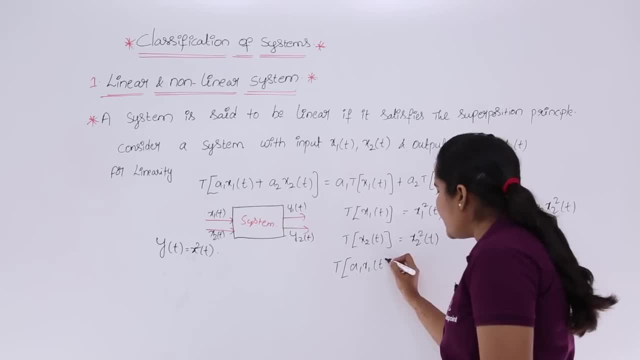 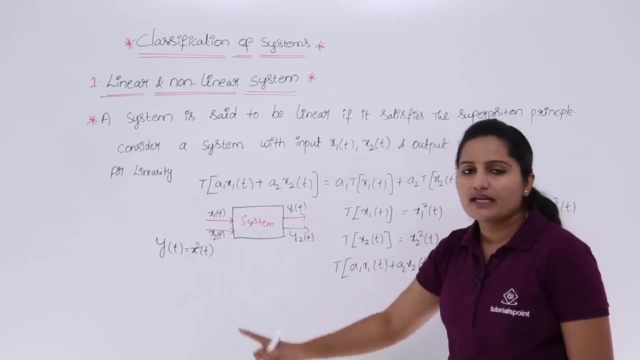 here. if you transformed the combined signal, that means a 1 x sum of t plus a 2 x 2 of t, then what system will do? system will do just squaring. why? because they, given that is a squaring system which squares the input waveform, it do not want what signal we are. 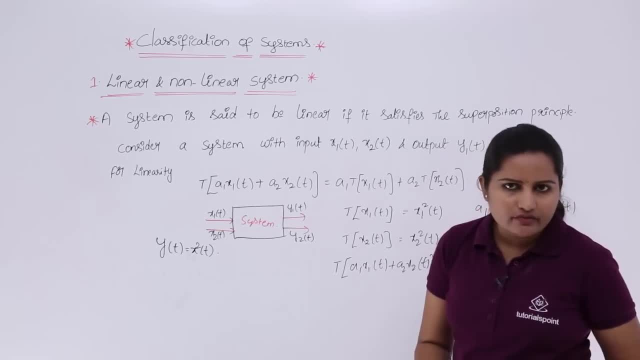 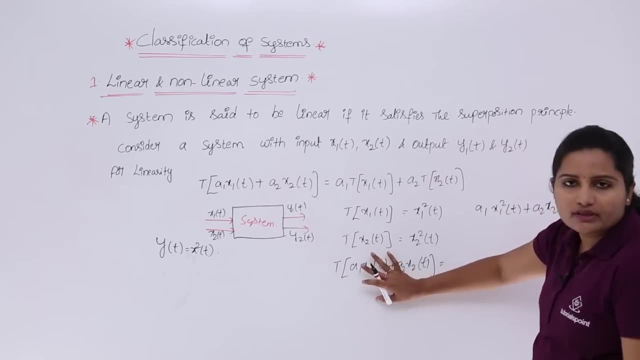 getting. That is a combined signal, that is a individual signal. whichever is signal that system is getting, that is going to square. So here that system, what, what is? what signal we want to transmit through that system? the combined signal, So system, do not want that. 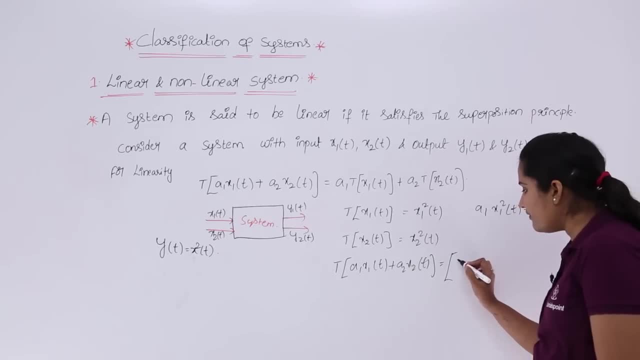 is a combined signal or individual, it is going to square whatever it is getting as input. So now, x 1 of t plus a to x 2 of t is going to square whatever we are giving in this transform. So so whatever we are having in the brackets, that means so that 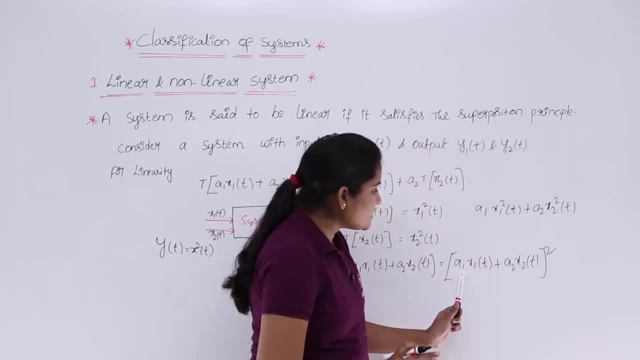 indicates, that is, we are giving to the system, So that system is going to square. So you can imagine these 2 are equal. So you can say these 2 are equal. no, we cannot say these 2 are equal, because this is just a 1 x 1 square of t plus a 2 x 2 square of. 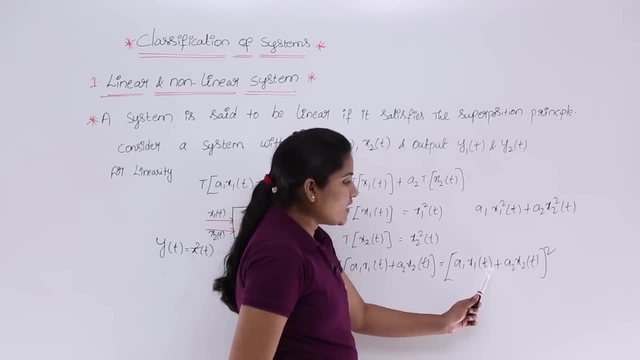 t, but here. so a 1 x 1 of t plus a 2 x 2 of t, whole square means. so a 1 x 1 of t plus a 2 x 2 of t, square will come, but plus 2 a b path, So that 2 a b path. so we are not going to get. 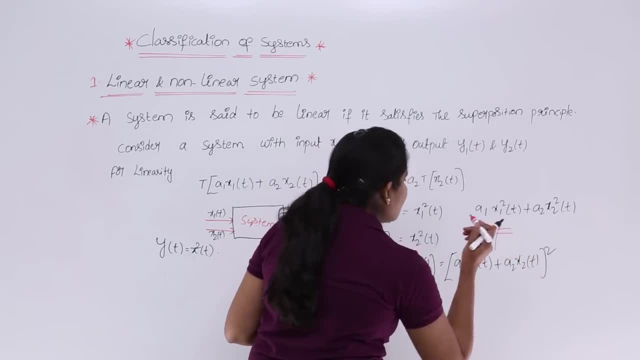 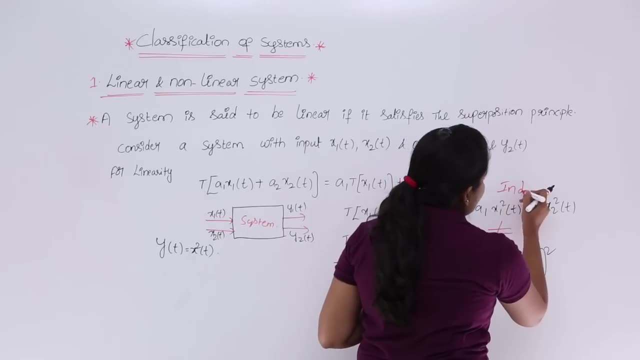 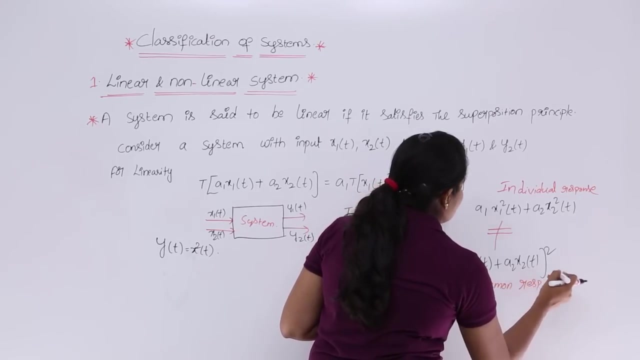 So here these two are not equal. that means it is violating superposition principle. that means this is a individual, individual response, this is a individual response, but here this is common response. So common signal response. So here as individual response is not equal, 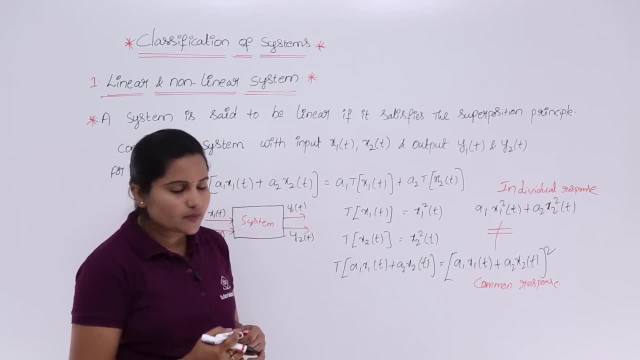 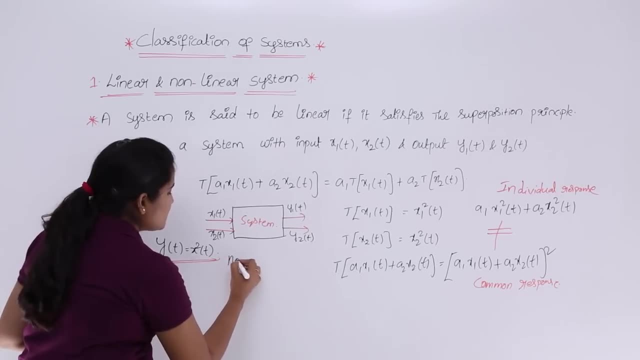 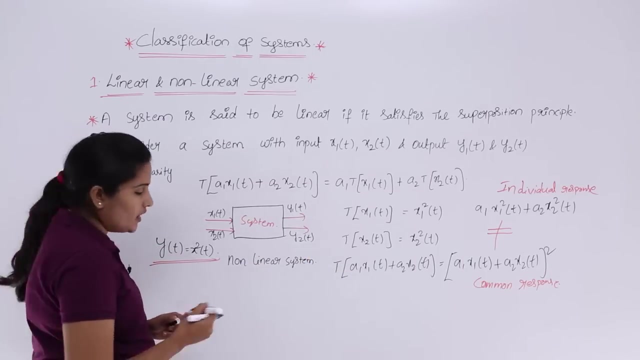 to common response. So it is violating superposition principle. So we can say: the system with this response is a non-linear system, this is a non-linear system. this is a non-linear system. For example, if you are having any non-linear 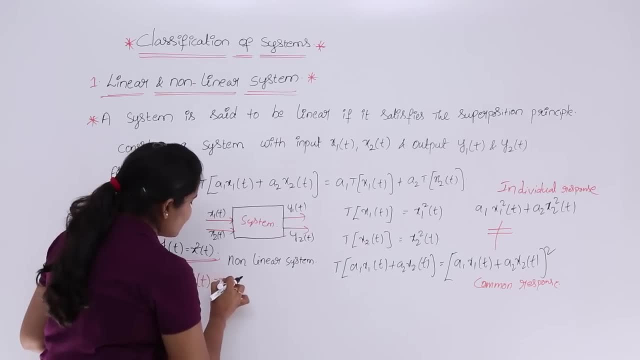 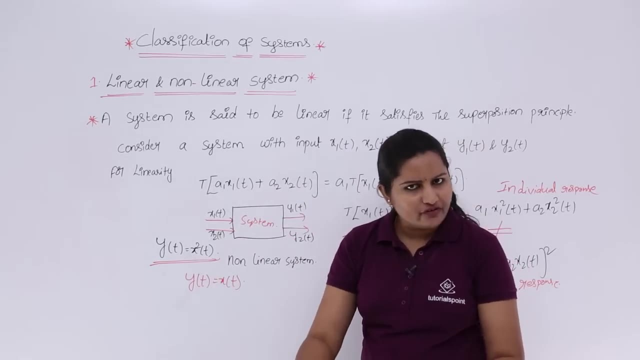 any system with y of t is equivalent to x of t. So this you just treat like a buffer. for example, you are having a system only with a buffer. it is. it may have some delay, but whatever signal we are giving, it is processing as usual. that means y of t equal to x of. 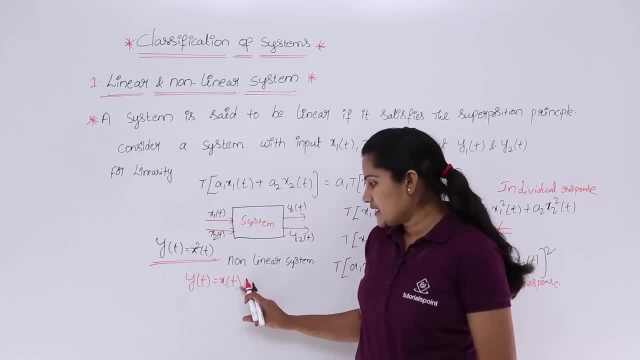 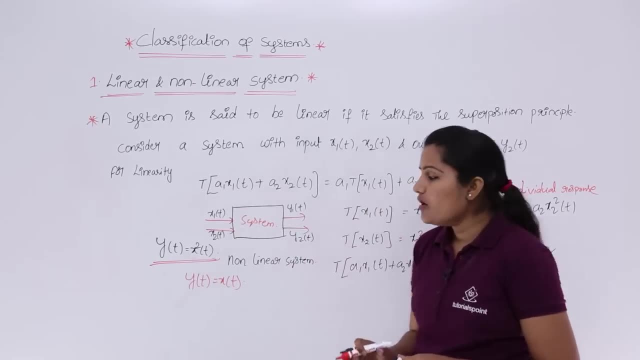 t is the response of a system. The response indicates whatever signal we are giving. same thing we are getting as a output. that is the meaning of y of t is equivalent to x of t. So now For this type of system. So that is a linear system or non-linear, if you want to check. 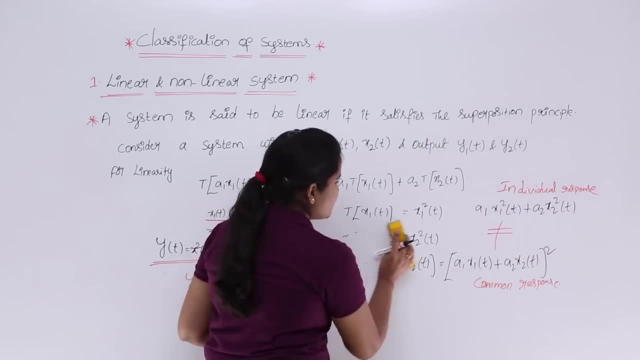 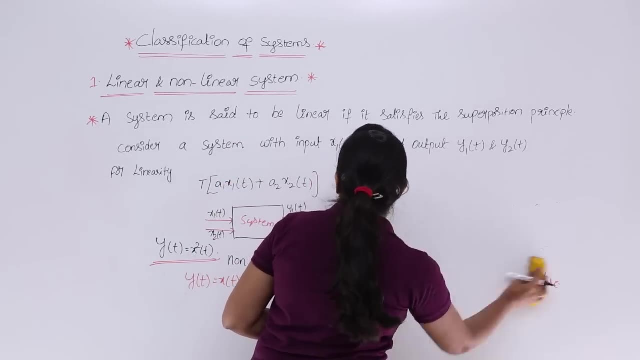 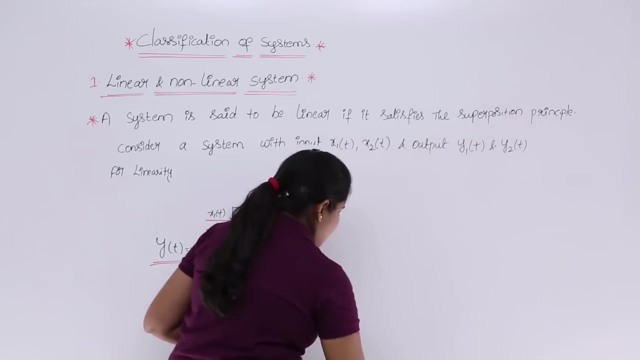 then, for example, if you given: I want to check that So you can see. So, first of all, what we need to check means we need to check whether the individual is equivalent to common signal. That means I want to check transform of x, 1 of t. 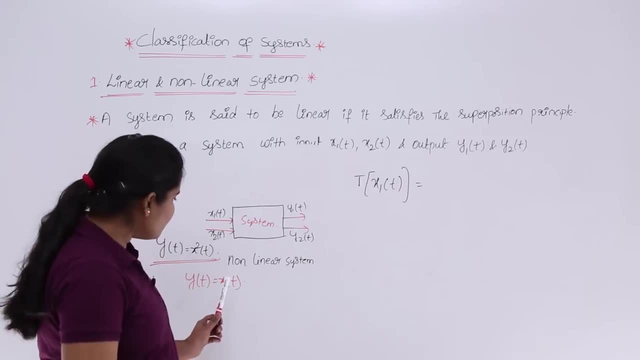 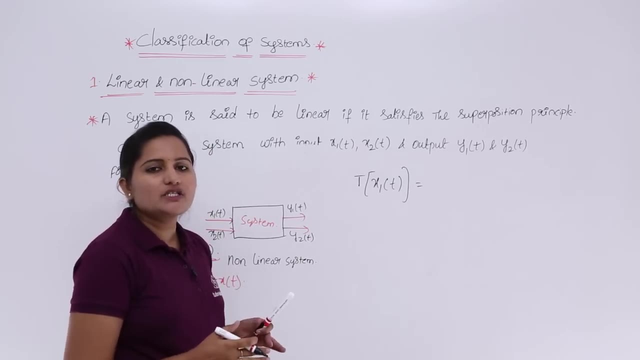 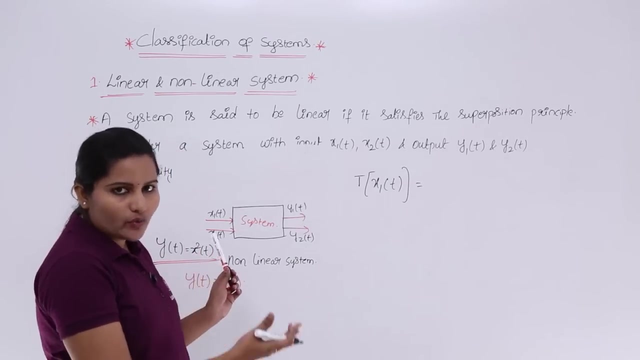 So here, transform of x, 1 of t signal through the system with this response will become x: 1 of t. only why? because now, in this case our system is going to process this signal without any change. but in case of last system we consider. So that is quiting. but here: 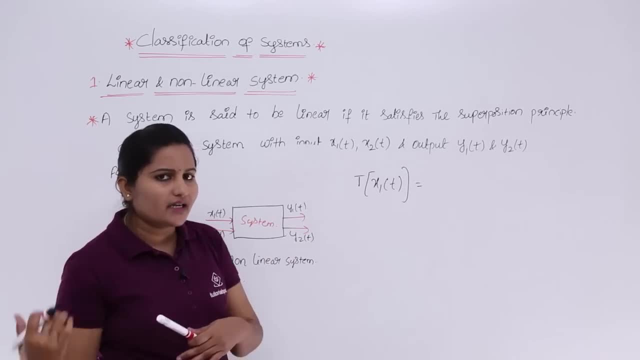 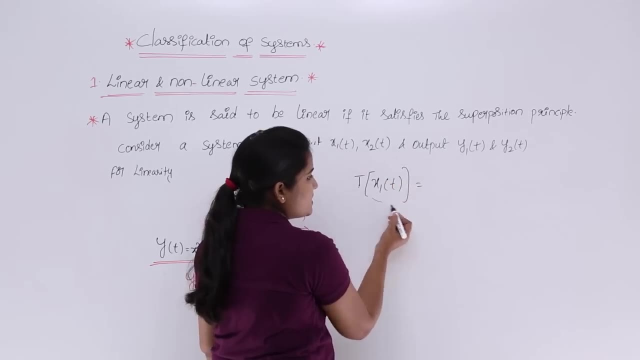 system is not doing anything, just processing whatever its getting as input. its just processing to the response or output. So if we given x 1 of t, if you want to transform this signal, signal to the ah- through the system, then the system is giving x 1 of t, only it is not going. 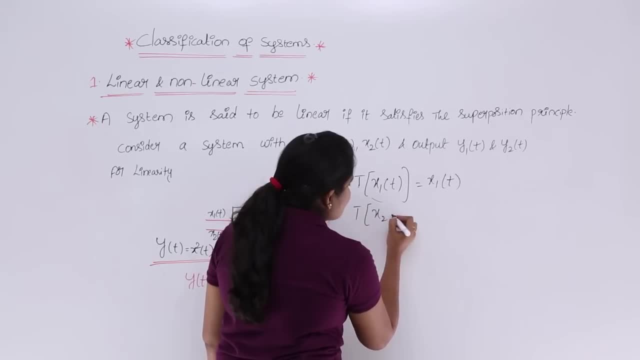 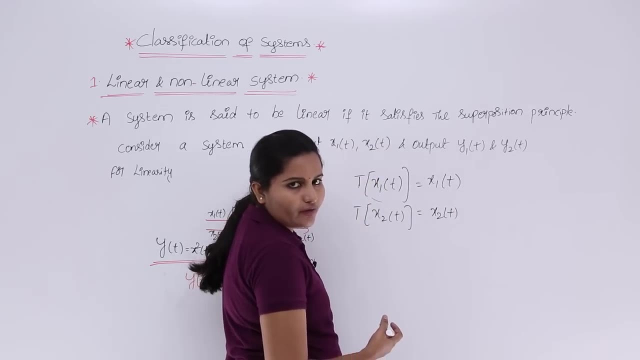 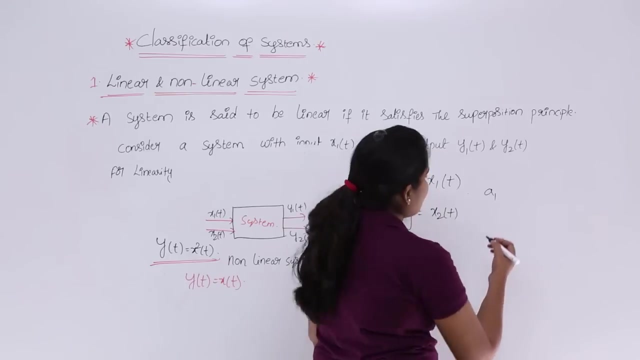 to change anything. So now, if you want to give x 2 of t also, it is going to get x 2 of t only. So if you consider the left part of ah, your superposition theorem, So this is equivalent to total response of system. for this, 2 signals is equivalent to a 1 x. 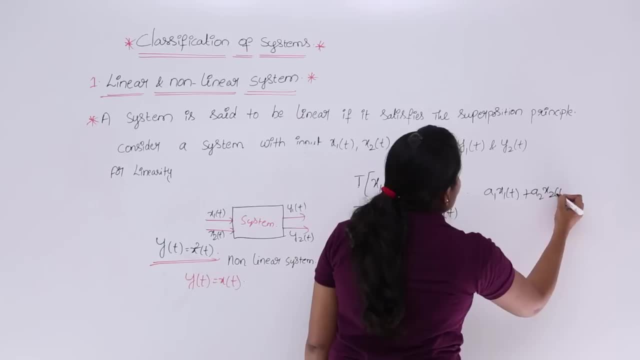 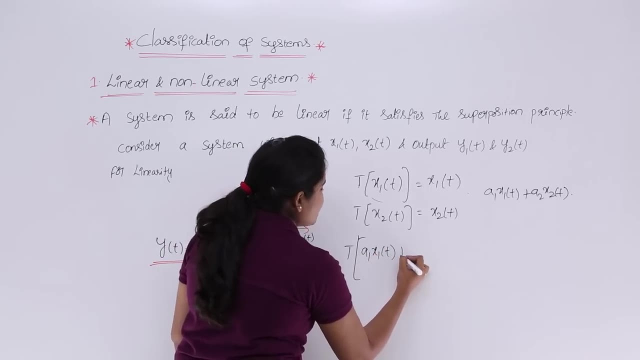 1 of t plus a 2 x 2 of t. So similarly, for example, if you consider the combined signal, that means a 1 x 1 of t plus a 2 x 2 of t. If you consider the combined signal with some. 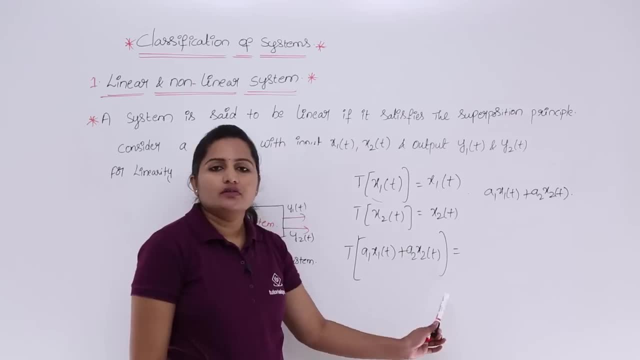 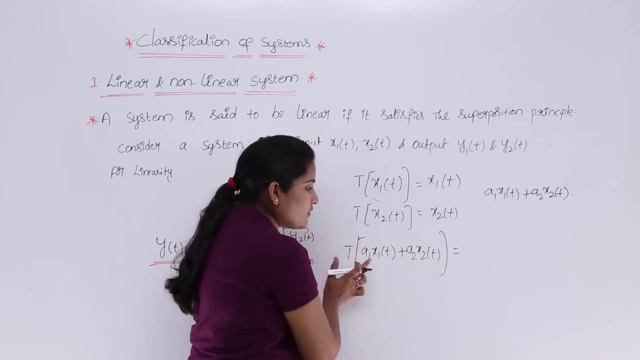 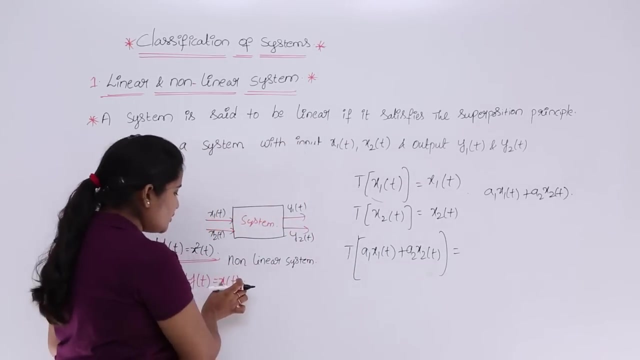 amplitudes like this, then here also system do not want whether we are giving combined signal or anything. So whatever we are giving to transform through that system, So according to our system response, it is going to change. So now our system is going to process. whatever we are giving, same thing it is going to process. 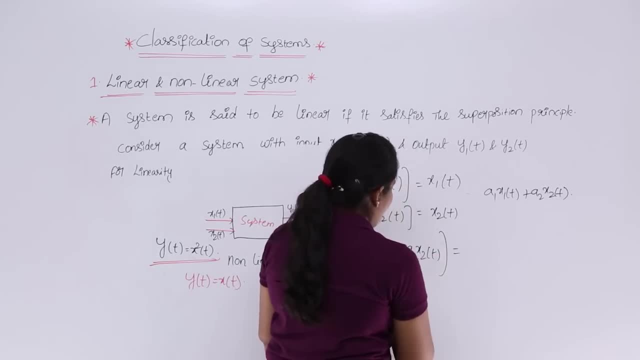 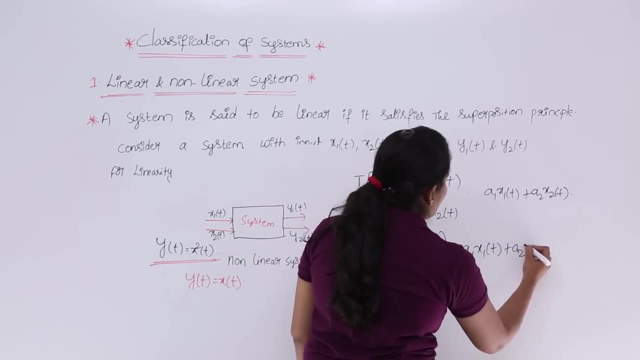 it to the output. So now here. so output is as same as we are giving. So that is equivalent to a 1 x 1 of t plus a 2 x 2 of t. So you can see- so this is individual response- that 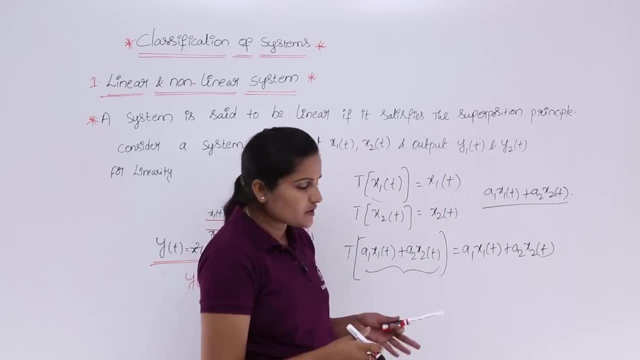 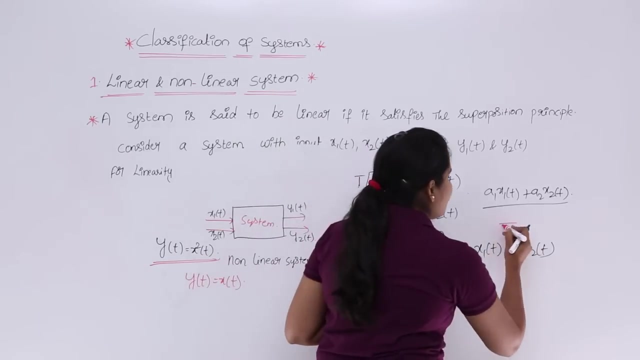 means combining of these 2 with amplitudes and this is common response. after combining signal. that means before giving as input we are combining Here individually we are giving and after getting response responses we are combining. So these 2 are equal. So